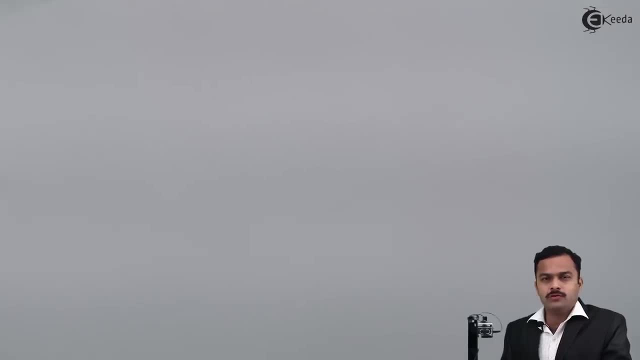 Hello, friends, in this video we are going to see the most fundamental law, along with Ohm's law, that we are supposed to use to solve a numerical. Not only a numerical, but lots of concepts are based on this law. So the law is Kirchhoff's voltage law, also known. 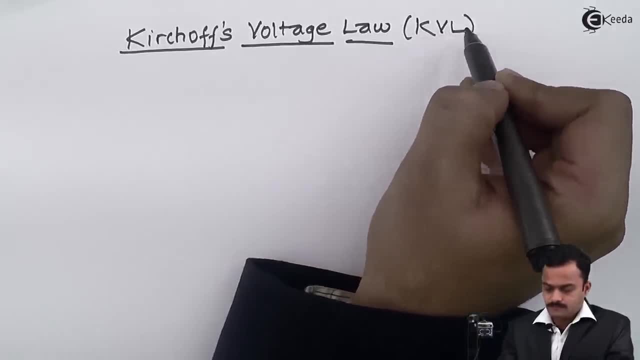 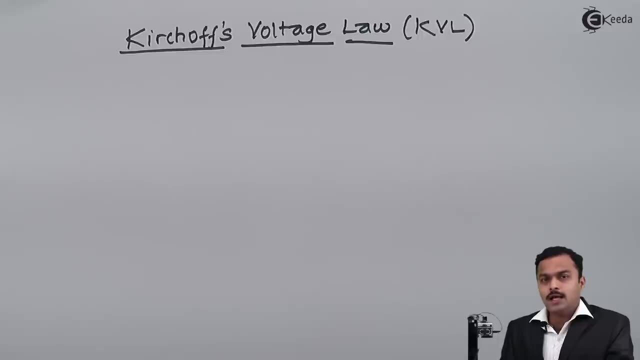 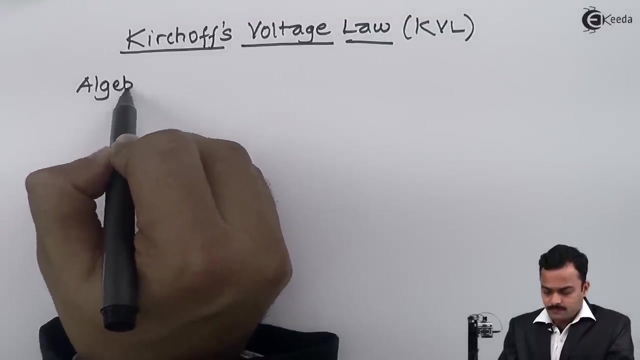 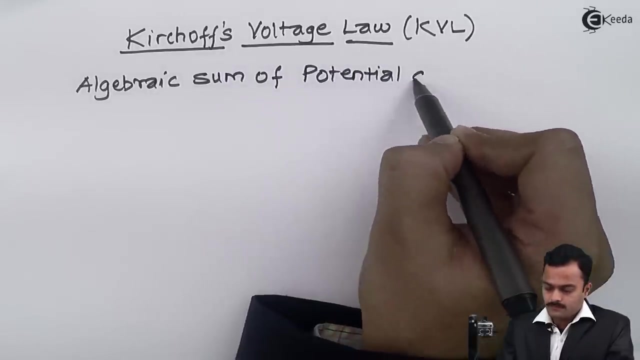 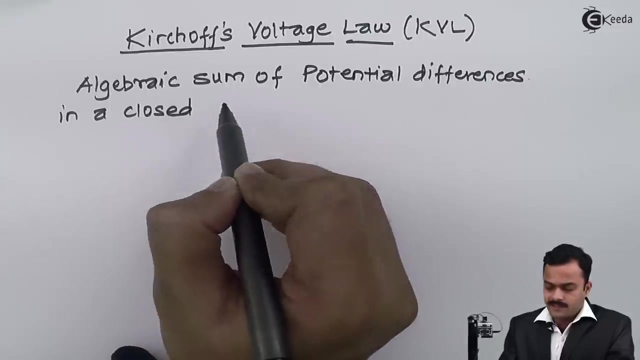 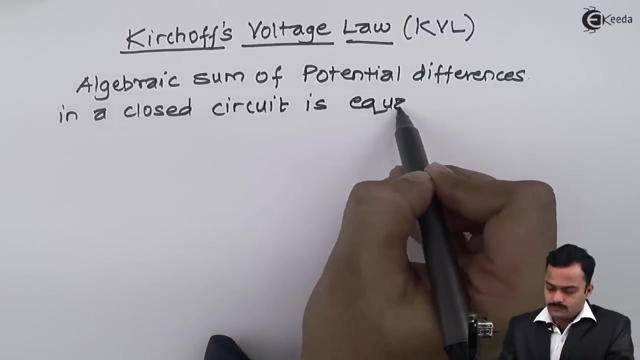 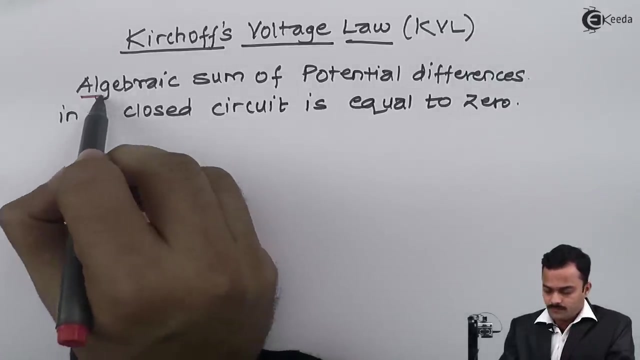 as KVL Law states that algebraic sum of all the potential difference in a loop is always equal to 0. So I repeat, algebraic sum of potential differences in a closed loop circuit, in a closed circuit, is equal to 0.. Again, the important concepts over here: algebraic. 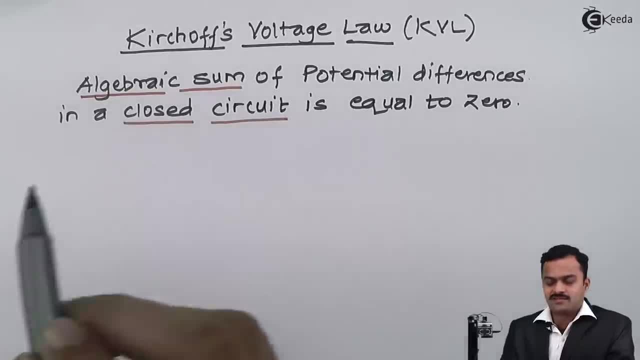 sum and what is the meaning of closed circuit? So to elaborate this, I will consider a simple circuit like this. So to elaborate this, I will consider a simple circuit like this. So to elaborate this, I will consider a simple circuit like this. 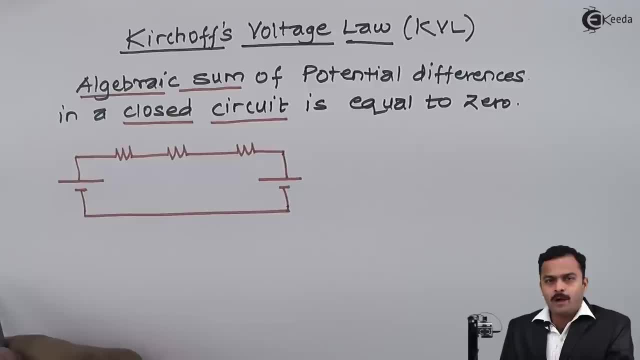 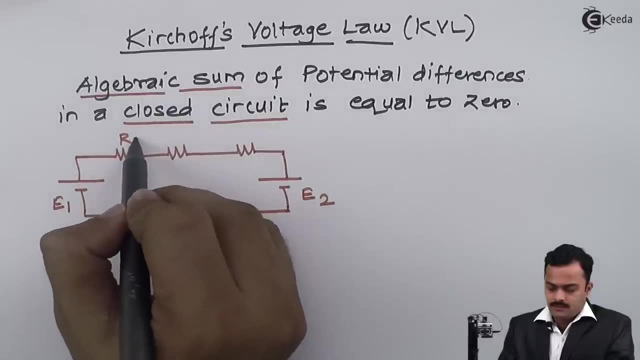 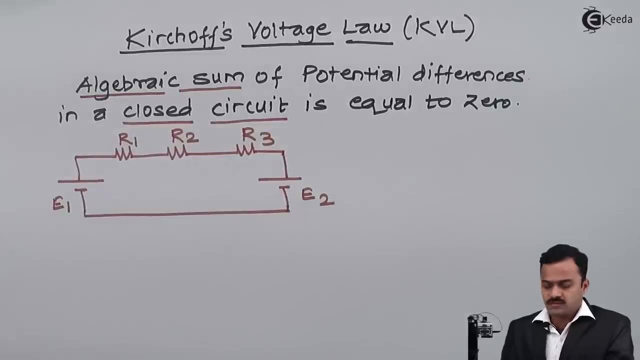 So I am having two batteries and three resistances connected in series like this, So obviously it is a closed circuit and current will flow and because of So I am having two batteries and three resistances connected in series like this, So obviously. 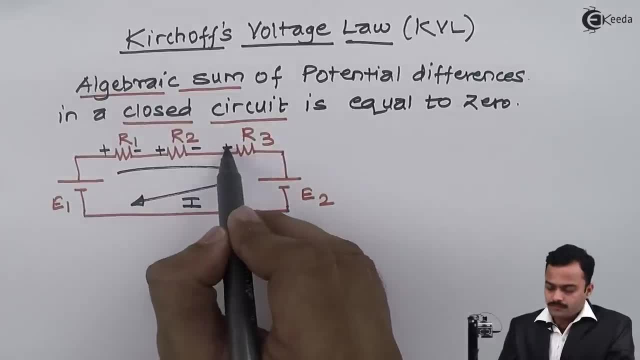 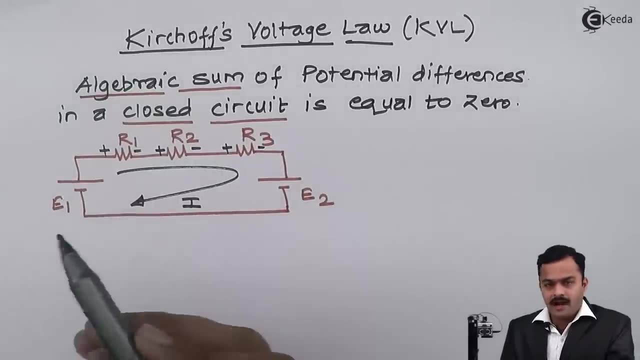 potential drop or voltage drop across these three resistances. Anyways, these are the batteries having fixed polarities like this. So we have to elaborate the concept of algebraic sum of potential differences. So here in all i am having 1,, 2,, 3,, 4, 5 elements. Each element is having some or other voltage. 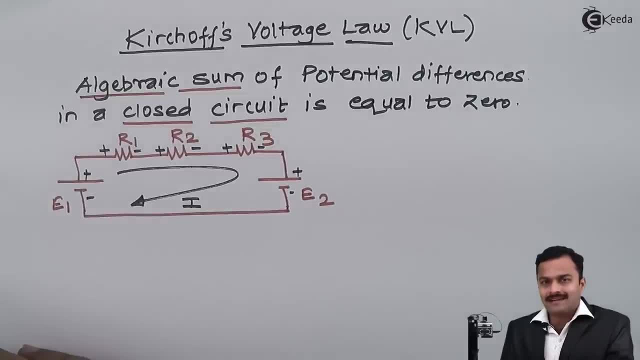 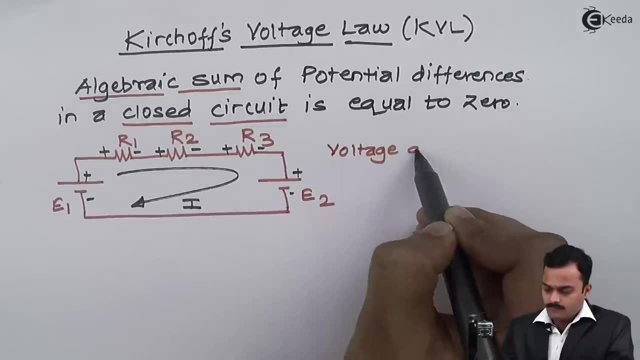 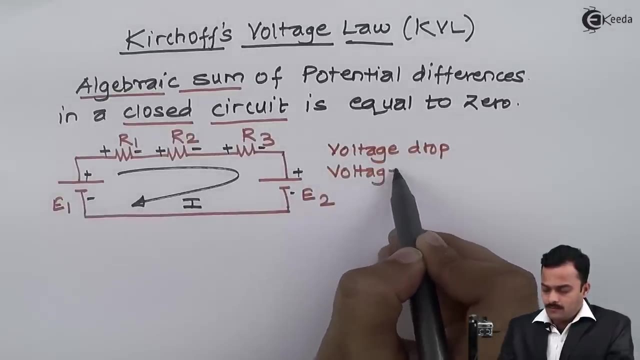 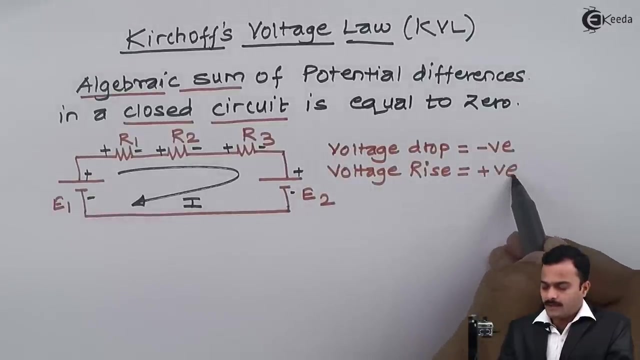 drop, or it can also be called as voltage rise. So I will write over here two concepts: voltage drop and voltage rise. So voltage drop I will consider as negative value and voltage rise I will consider as positive value. Now understand the meaning and difference between voltage. 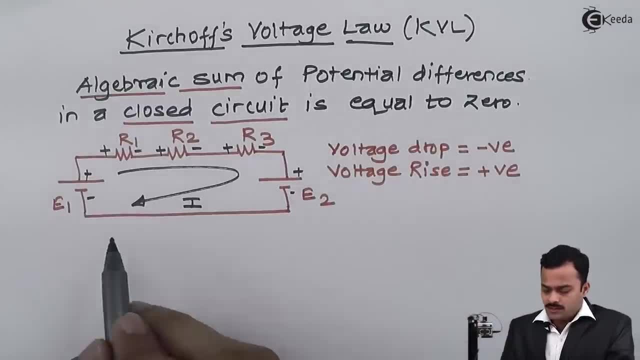 drop and voltage rise. Suppose there is one element connected between these two points. It could be anything, It could be a battery or it could be a resistance. and if in the direction of current. if the two terminals having the polarities plus, minus in the direction of current, meaning the polarity is changing from. 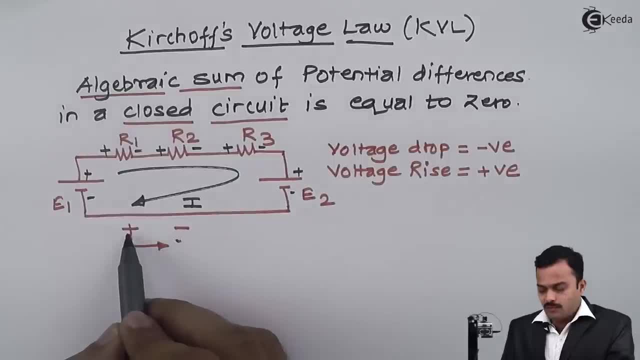 plus to minus. So whenever it is changing from plus to minus I will consider that particular potential as voltage drop. Likewise, if in the direction of a current or tracing, a closed circuit, if I'm having an element voltage polarity changing from minus to plus, it could be. 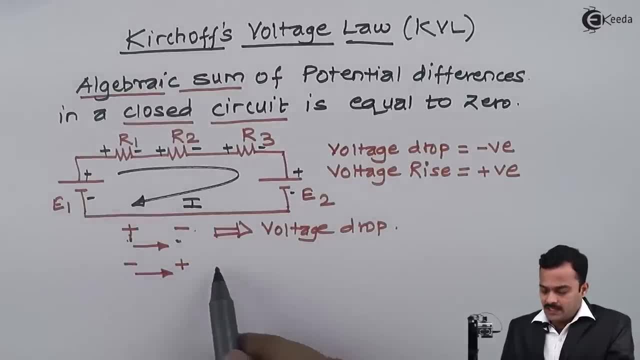 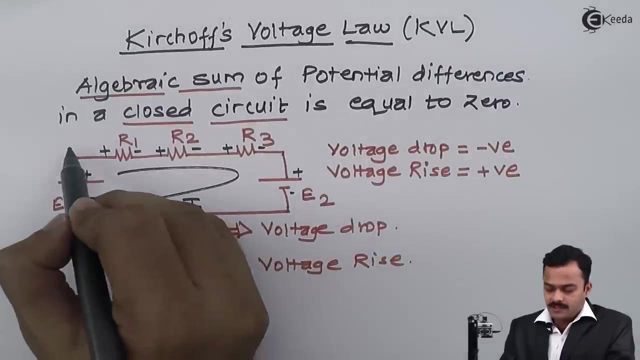 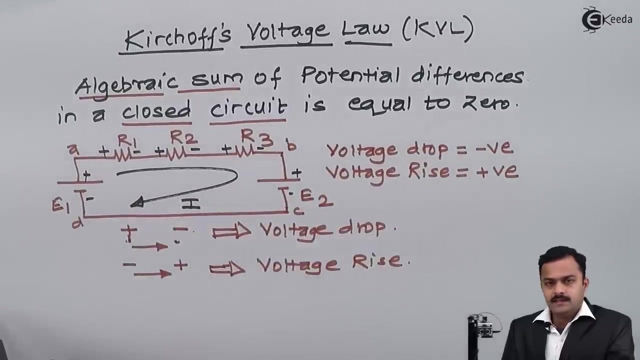 anything, either a resistance or a battery. I will consider that particular potential as voltage rise. So let's apply this concept to the circuit. Now I'm considering loop A, B, C, D and, if I, tracing a path from A, B, C, D back to 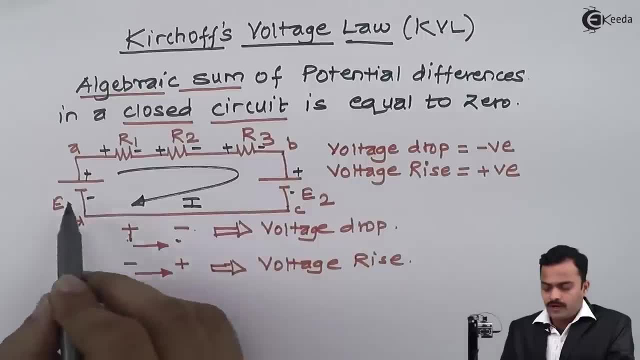 the A, I can have one, two, three, four, five potential differences, So let's start with R1.. So in this direction it is changing from plus to minus. Plus to minus I consider as a voltage drop. So in this direction it is changing from plus to minus. Plus to minus I consider as a voltage drop. 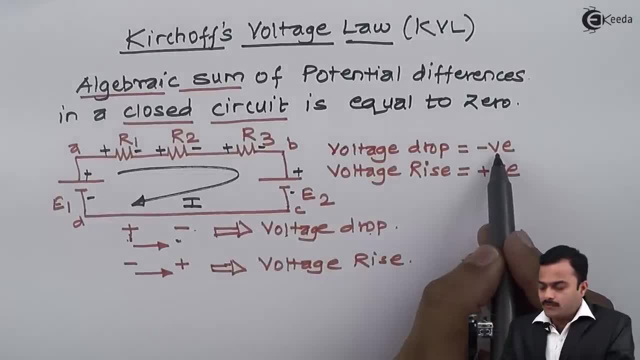 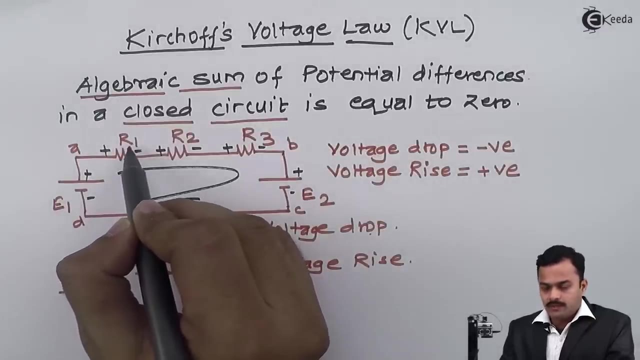 And I will consider that particular value as negative. So for this resistance, so voltage drop, I will write as minus I into R1.. Current flowing through the R1 is I. Resistance value is R1.. So I into R1 is a voltage or a potential, Same way for R2.. 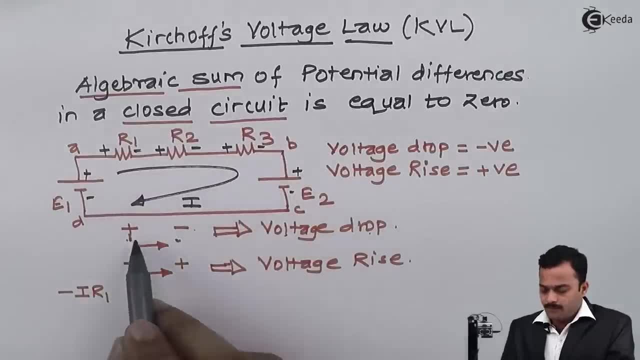 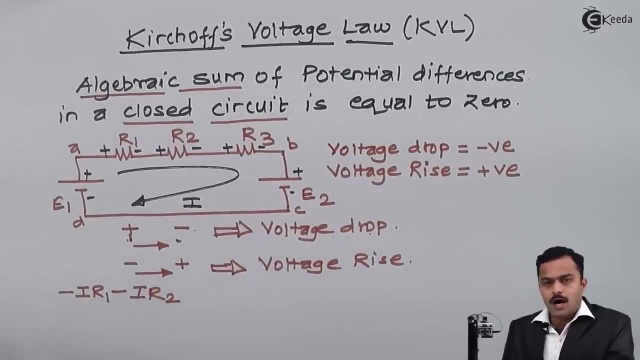 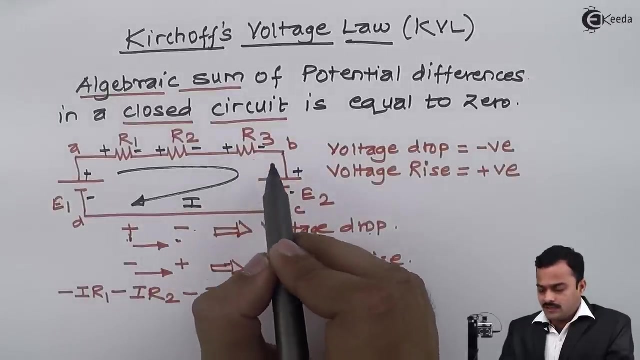 In this direction. I am having plus to minus. Plus to minus is again a voltage drop, which is a negative. So minus I R2.. Third, again a resistance having the same polarity plus minus. So I will get minus I R3.. Now pay attention, In the direction of current. here I'm tracing all the voltage drops like this: 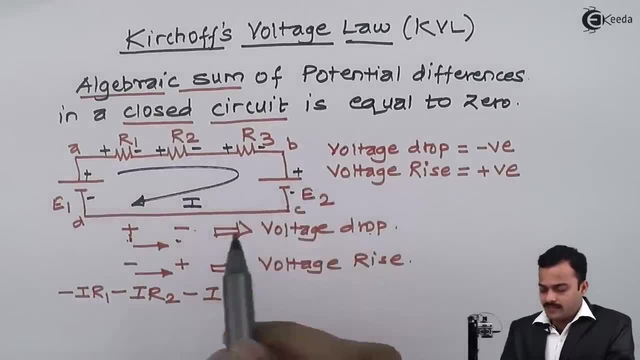 I'm having plus minus, Once again plus minus, So it's a voltage drop. But hold on, It is not a resistance, It is a voltage drop, But hold on, It is not a resistance, It is a voltage drop, But hold on. It is not a resistance, It is a voltage drop. 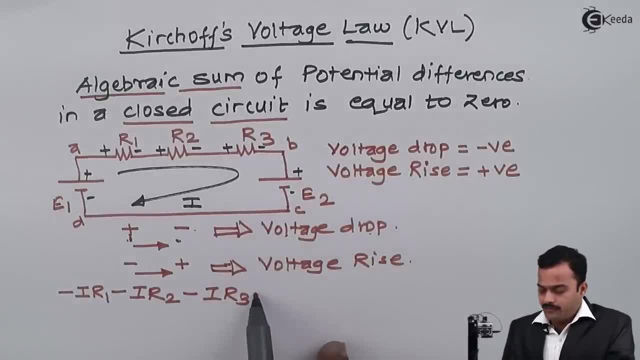 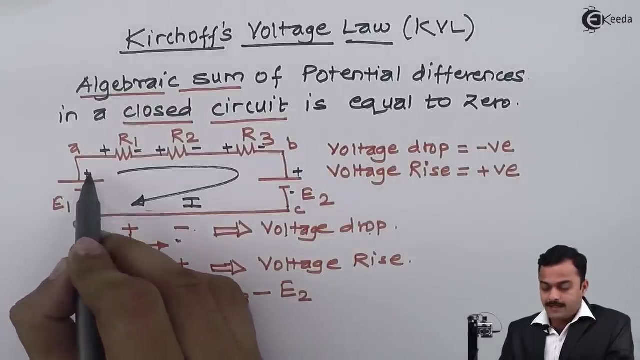 It is a fixed voltage battery, So I will have a minus sign because it is plus to minus, But I should not write I into E2.. In fact I should write only E2, because that is a fixed voltage I am having, irrespective of amount of current, And finally, in the direction of current I am having last potential as minus plus. 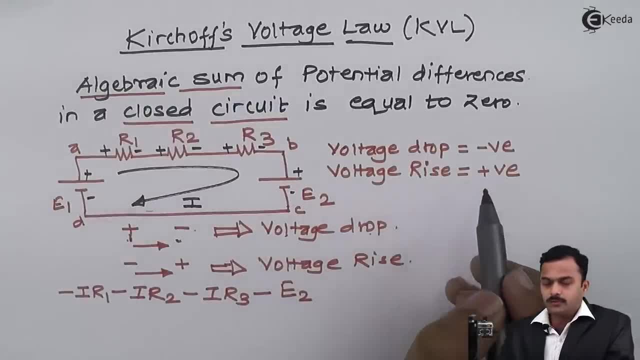 Minus, plus is voltage rise, So voltage rise should be denoted plus and, mind you, it's a battery, so it will have simply plus. e1 equals to 0. so ultimately I can say these two are the battery voltages which I can club. 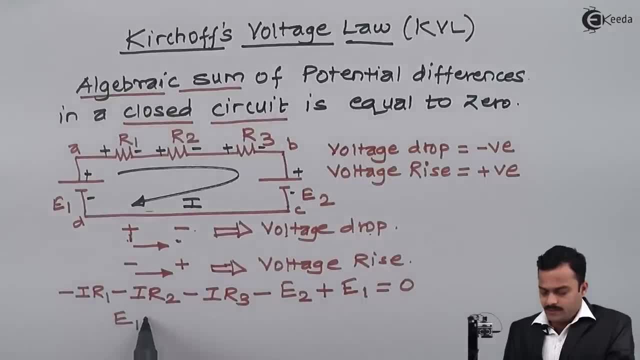 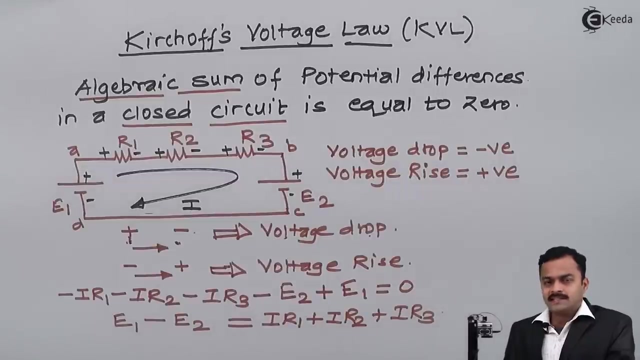 together e1 minus e2, equal to this. three IR1, IR2, IR3- are the voltage drops. so I can write here IR1 plus IR2 plus IR3. so ultimately what is happening, all the potential and amount of energy will remain conserved. so KVL can also be.